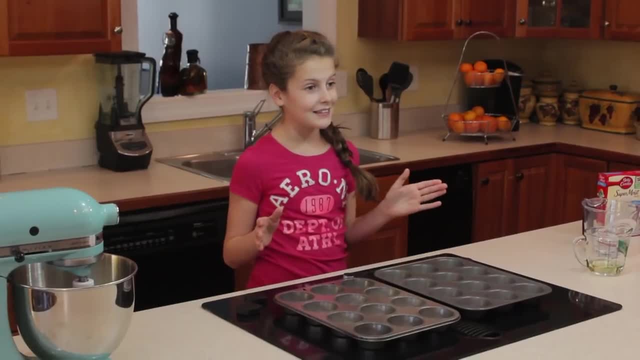 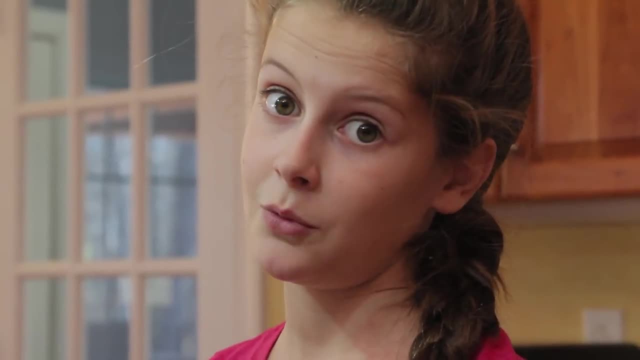 at it. it's super easy and I'll show you how to do it. Plus, I'm going to show you my own special twist to add to the cupcakes to make them more better-er-er-er. Yep, that's a word For this. 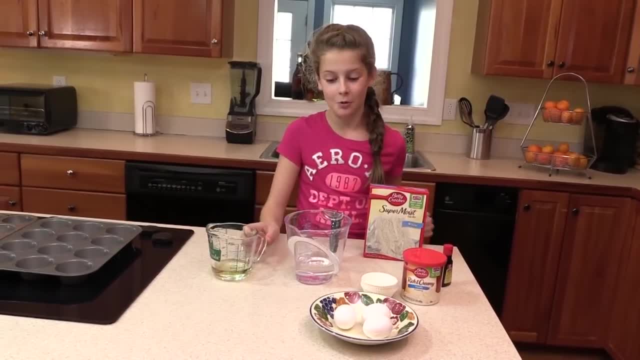 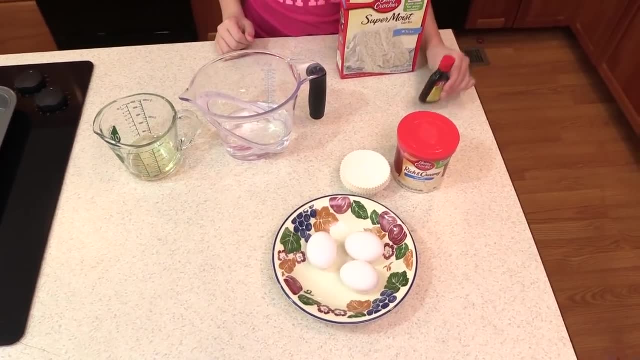 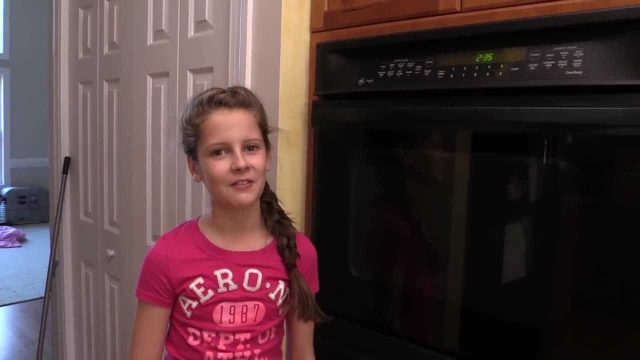 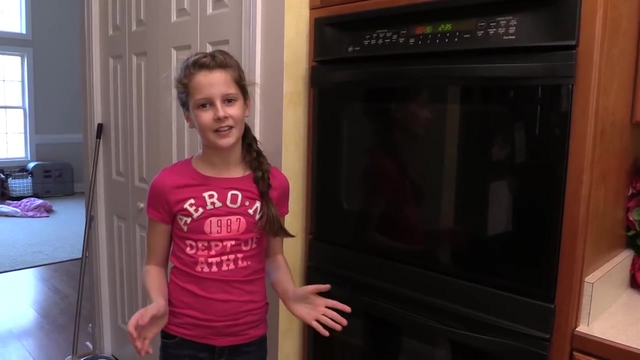 simple recipe. all you need is a third cup of vegetable oil, one and a quarter cup of water, three egg whites and my special twist almond extract. First, preheat the oven to 350 degrees. If you're not comfortable using the oven, ask an adult to help. 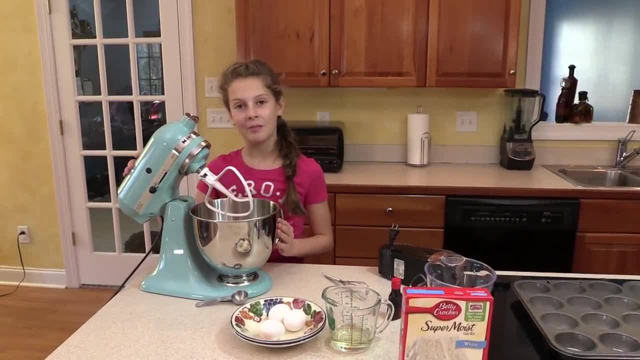 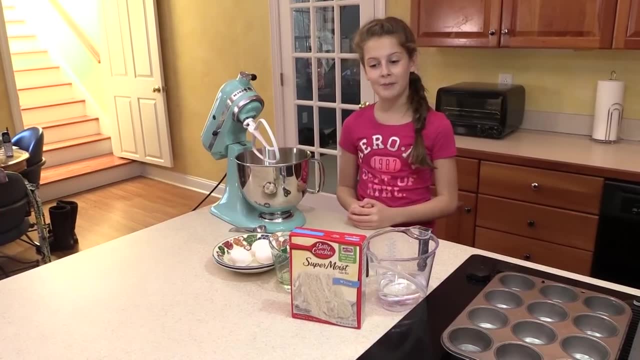 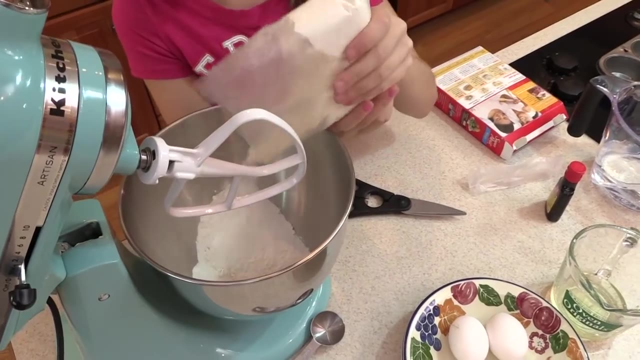 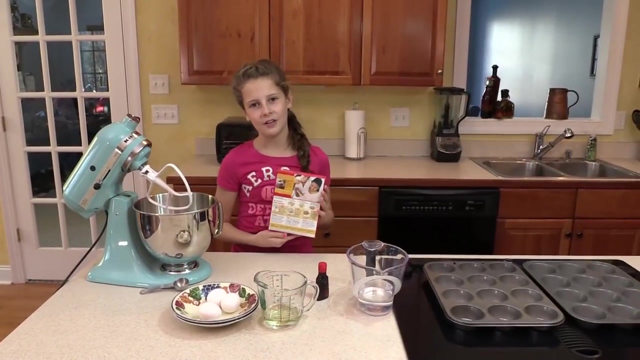 Now it's time to put the recipe together. I'm using my favorite mixer from Christmas, but you can use an electric mixer or even a whisk, It doesn't matter. Start by putting the cake mix in. Okay, so the directions are right here on the box. 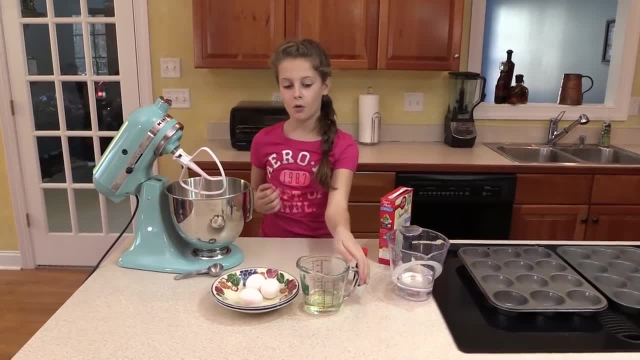 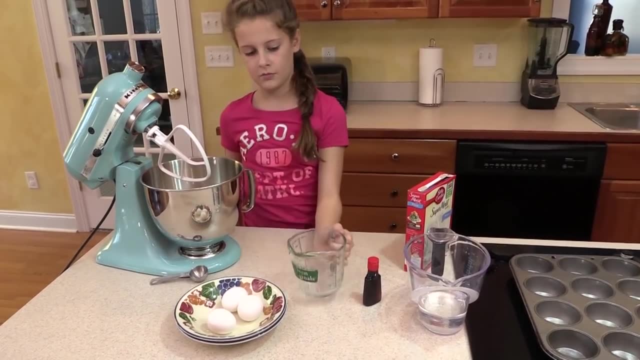 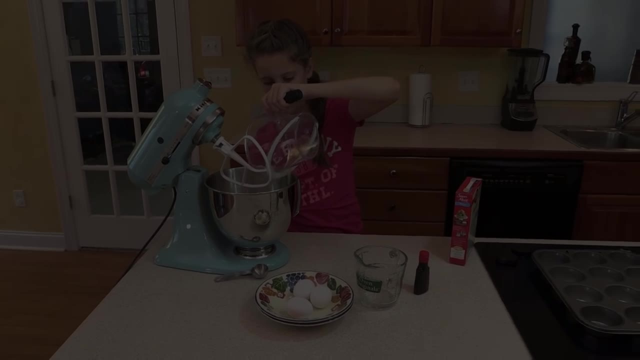 but I'm going to tell you what to do anyways. Next, you add the oil and the water. I'm going to add the milk and the egg whites and I'm going to add the milk and the egg whites. I'm going to add the milk and the egg whites and I'm going to add the milk and the egg whites. 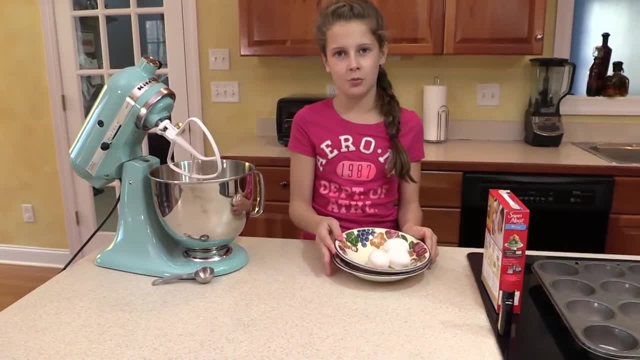 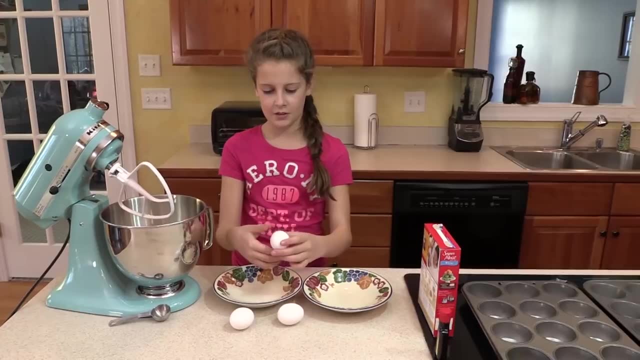 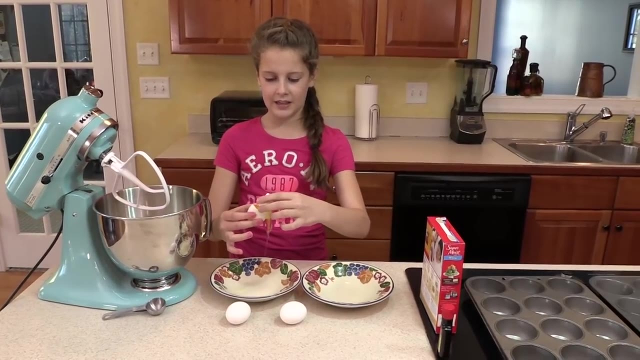 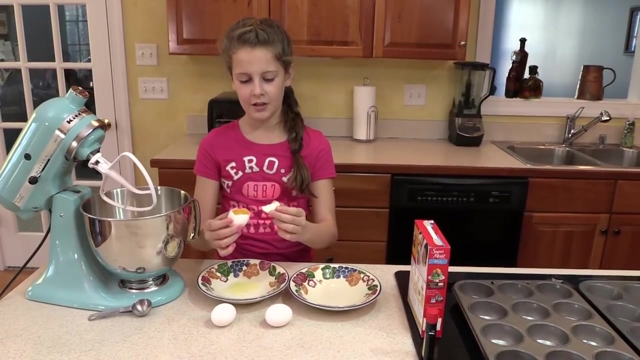 The trickiest part of them all is the egg whites. You're going to need two bowls, Okay, so just open an egg and crack an egg, like you normally would, and let all the egg whites that can spill out. Sometimes I use the top of the egg just to help get them out. 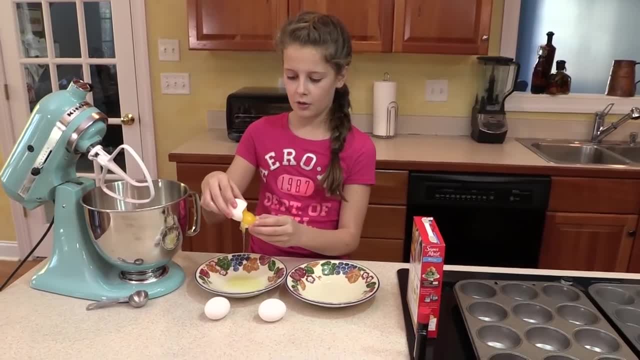 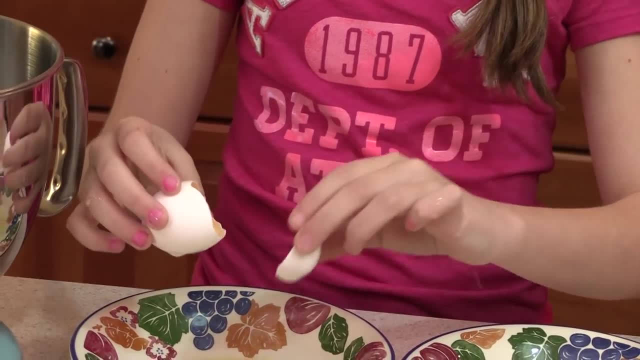 Now you try and pick up the yolk with the other part of the shell and let the rest of the egg whites spill out. Keep doing this until you feel that all the egg whites have come out and then put the yolk in a separate bowl. 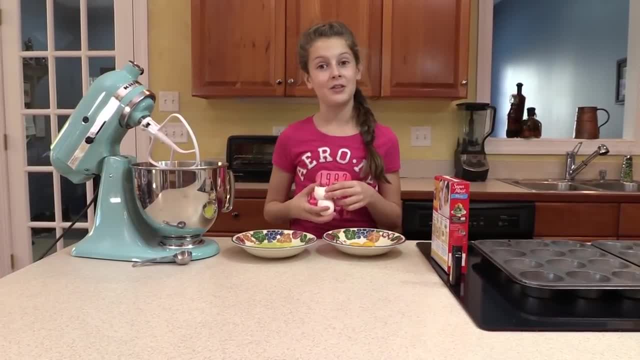 Make sure you wash your hands after handling eggs, because raw eggs can make you sick. Okay, so I'm going to add the milk and the egg whites and I'm going to add the milk and the egg whites. Okay so, I'm going to add the milk and the egg whites and I'm going to add the milk and the egg whites. 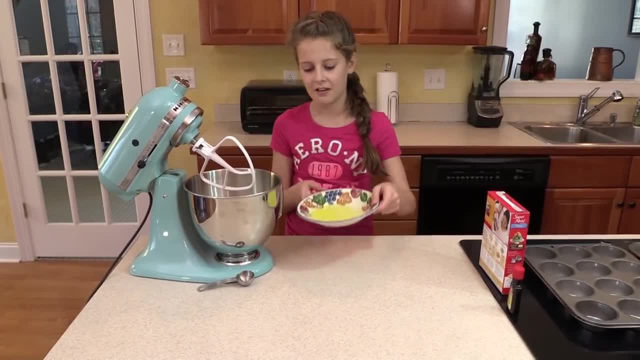 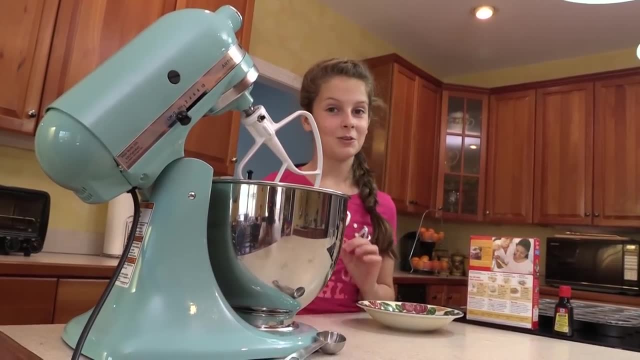 Okay, we got rid of the egg yolks and the shells, so now just add the egg whites to the mix. Now it's time for the special twist Almond extract. Trust me, it's great. All you need is about a tablespoon. 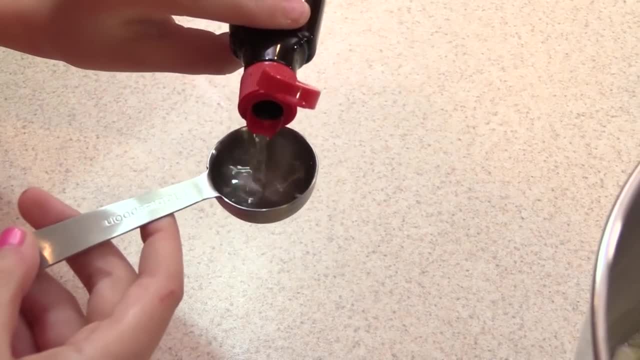 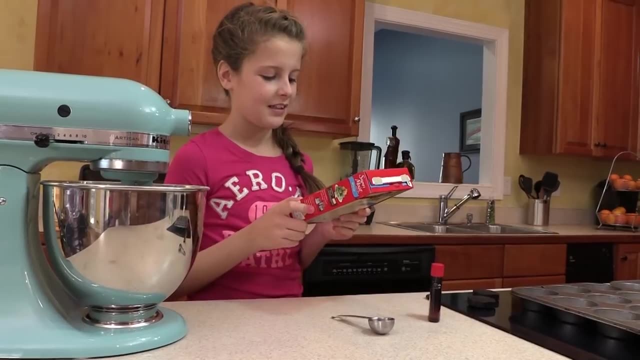 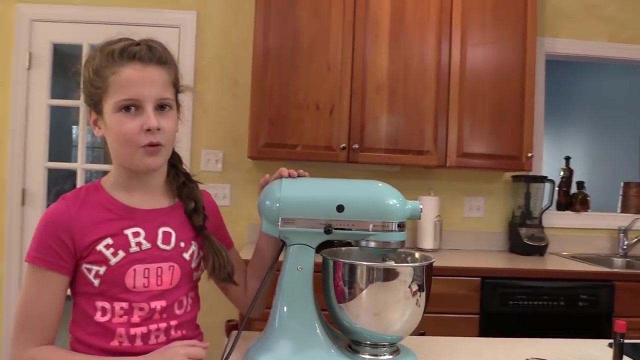 Careful it comes out kind of fast. Beat on low speed for 30 seconds, medium speed for two minutes. I never do that, just put it in the mixer and put it on medium speed until a batter forms. it'll be a little bit lumpy. 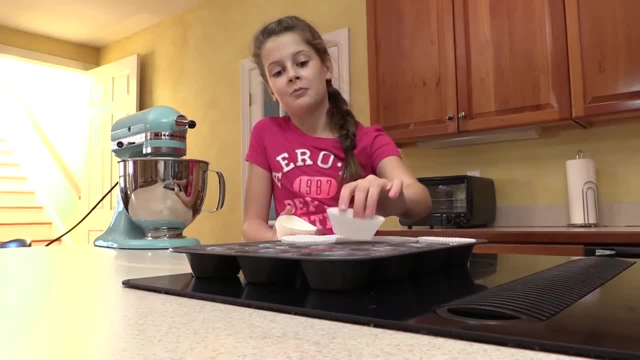 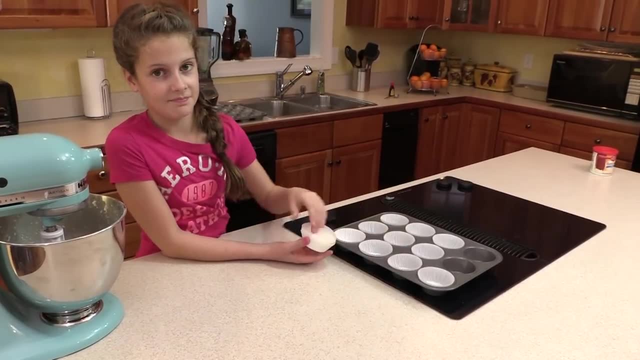 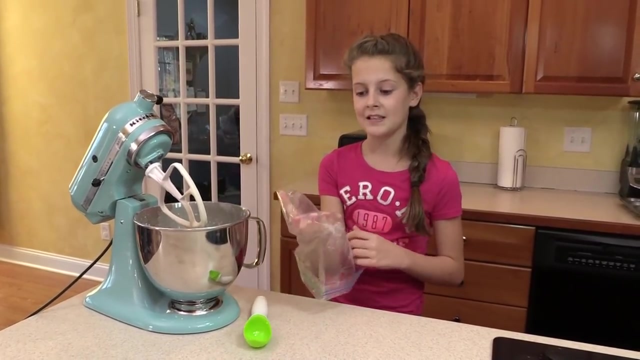 it may seem obvious, but cupcake liners make your life a whole lot easier. they come in all different colors and they make cleanup so much easier. here's a helpful tip to avoid messes and to get the cake batter into the pan. so you take a regular ziploc baggie and put it inside out with your hand inside of it. 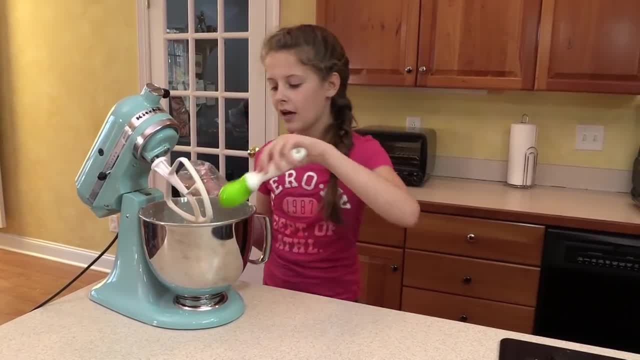 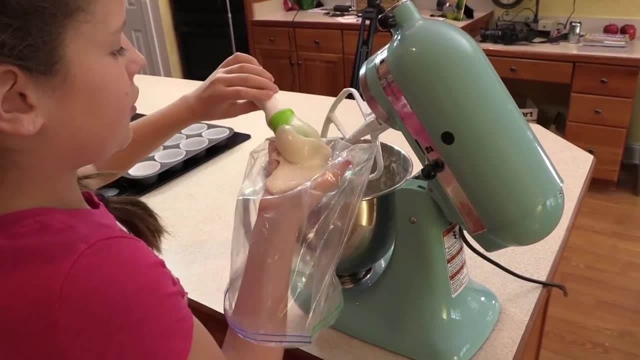 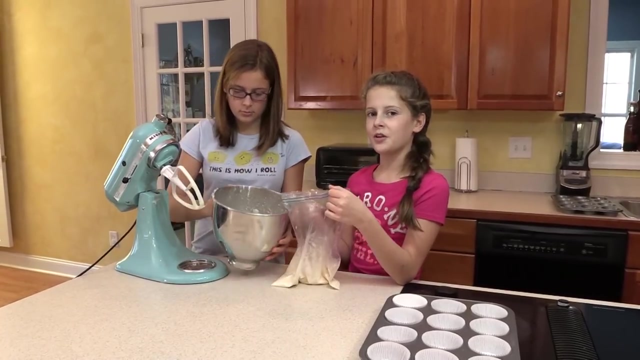 yeah, you just get a spoon- I'm just using an ice cream scooper- and you scoop it into your hand like this. just do this for in little chunks, or however much you want to do. if you don't have time to do it scoop by scoop, ask someone help to. 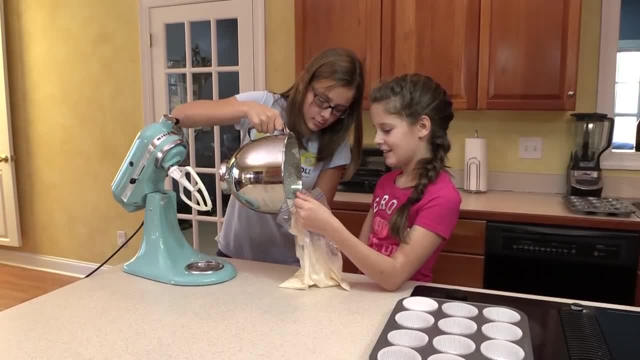 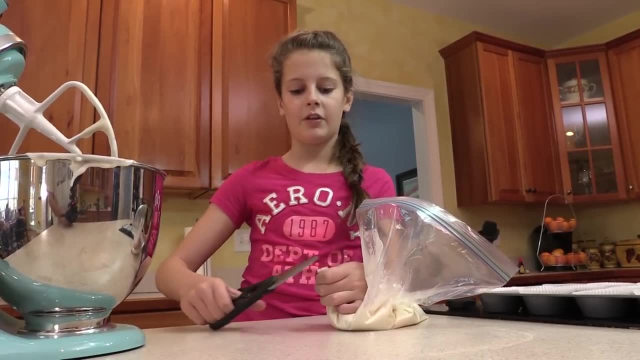 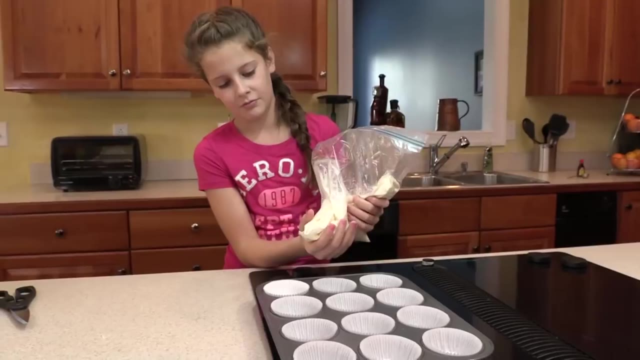 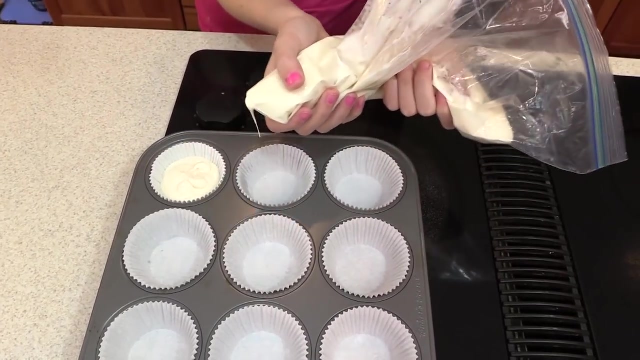 help you get it in there. thanks, Mary. next, you want to pinch a little corner of it of the bag and cut, cut a tip off with scissors. so then you hold the bag with like this, or however you is comfortable for you, and fill the cupcake liners about two-thirds full. do this for. 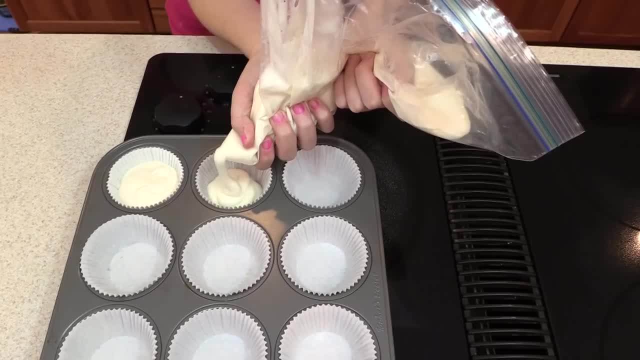 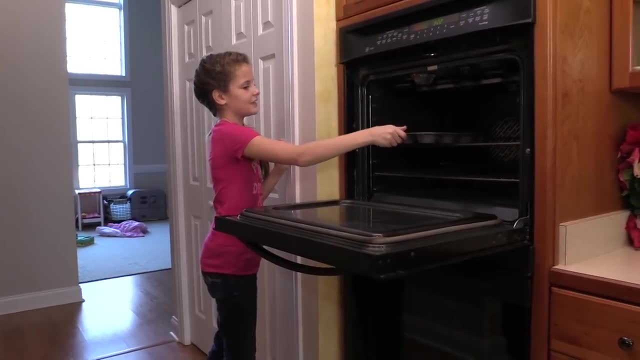 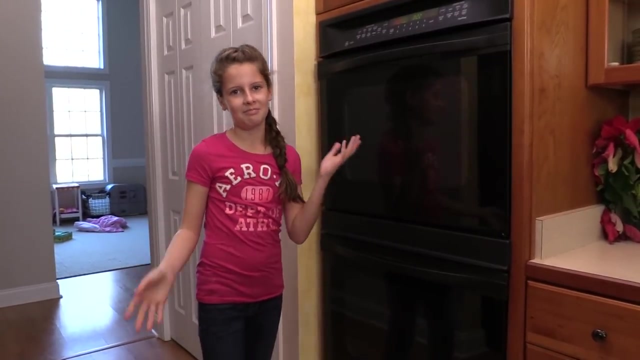 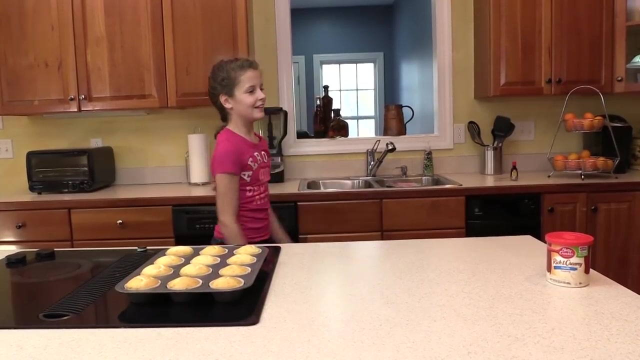 the rest of the cupcakes. now it's time to put the cupcakes in the oven. let them bake for about 20 minutes. you see, I could probably use the time wisely and go clean my room, but I'll probably just get on Instagram. these cupcakes look pretty great. check right here for an awesome decorating video. go ahead. 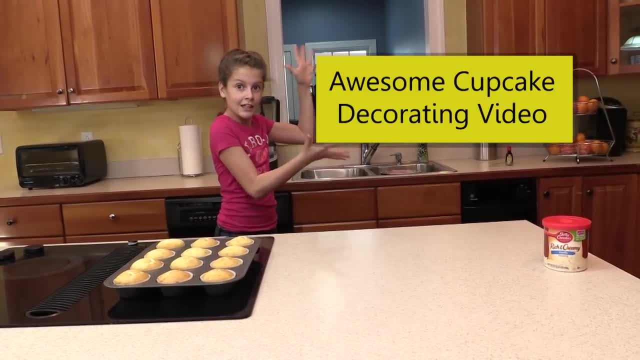 click it. you know you want to.